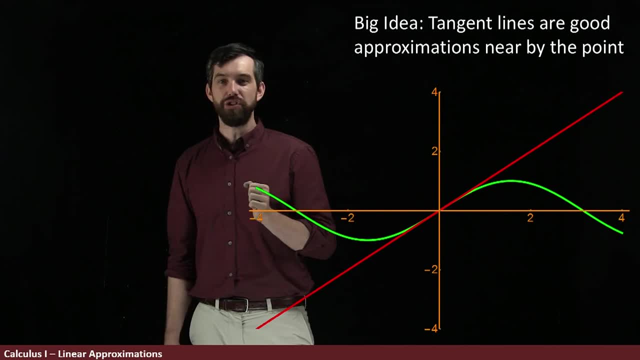 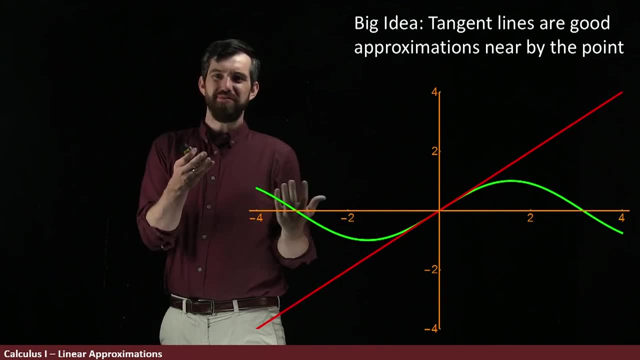 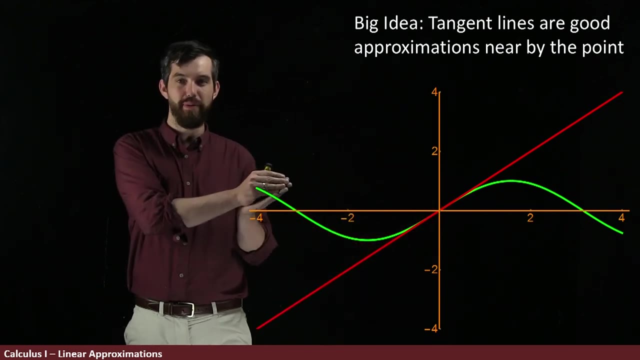 And what I've computed for you is the slope of its tangent line at x equal to 0. So I've got some particular line and I computed this by the derivative of sine of x And you can sort of intuitively see here that right near 0, sine and its tangent line are like right on top of each other. 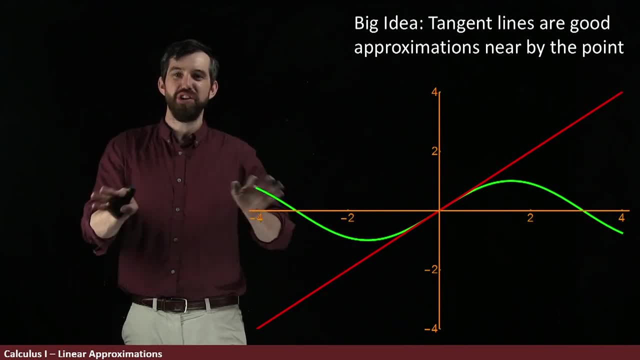 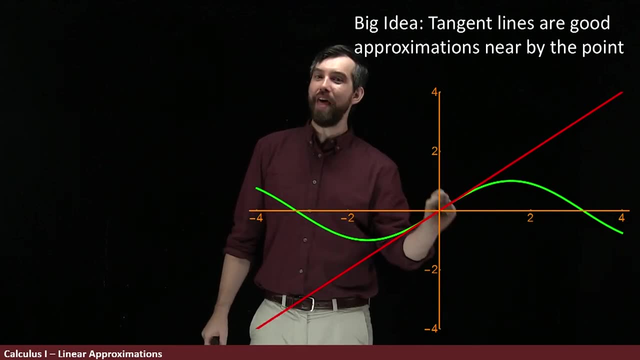 But far away, like over here, sine and the tangent line have nothing to do with each other. It's quite dependent on the fact that the tangent line is a tangent line. at one point And near that one point where I put my tangent line, it's a pretty good approximation. 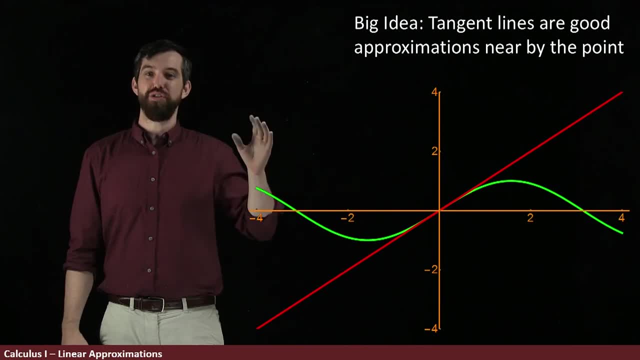 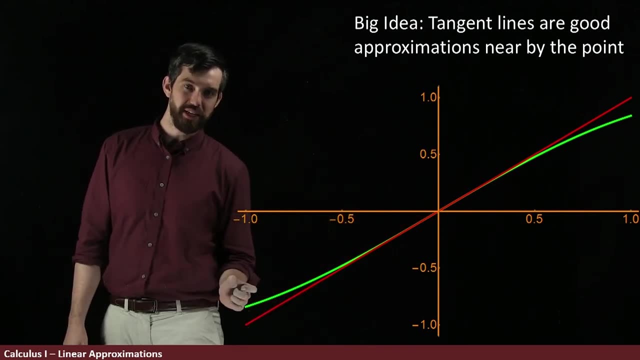 Far away. it absolutely does not appear to be. I'm going to do sort of imagine, I'm going to zoom in here a little bit. So I've now narrowed my window. now It's only minus 1 to 1 here, And you'll notice that it looks good for longer. 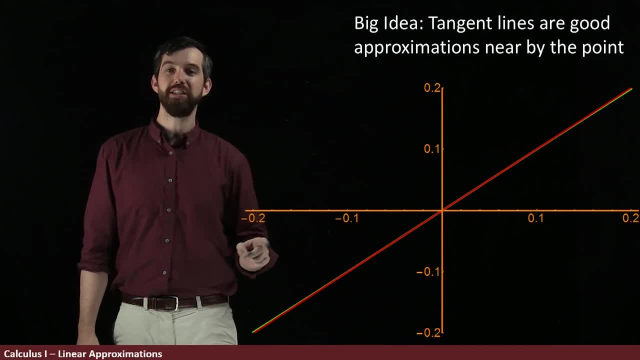 Okay, let me zoom in again. Minus 1 to 1 is what I have right now. Now I'm going to go minus 0.2 to 0.2., And I don't even know if you can resolve this on your screen. 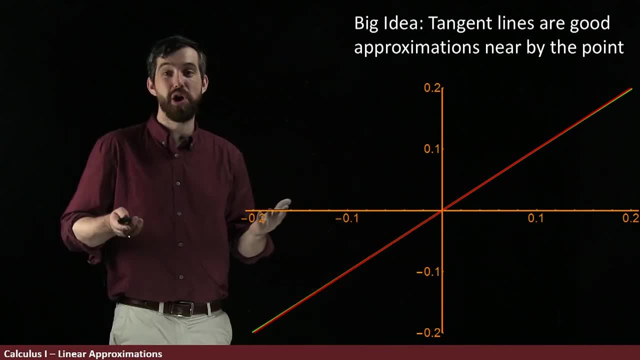 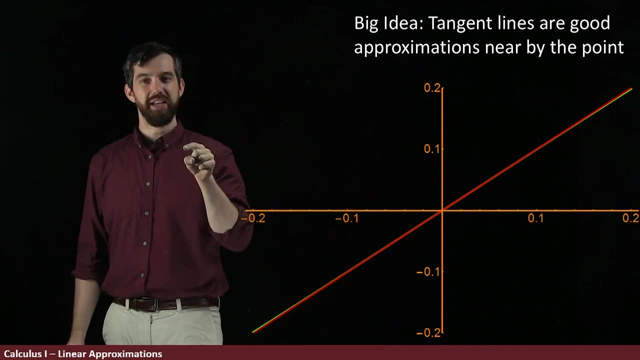 The red and the green, the sine and its tangent line are basically on top of each other as I zoom in on that window. So if I zoom in close enough, the tangent line and the equation, the original function here, appear to be almost interchangeable. 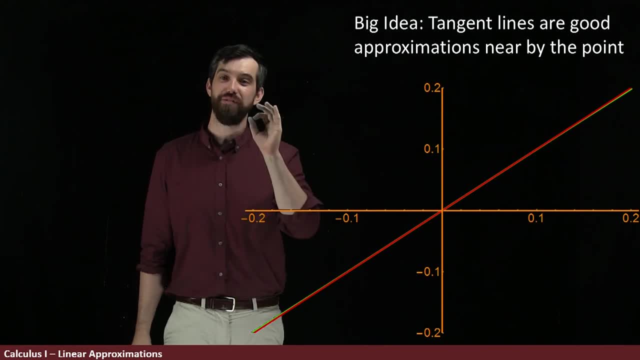 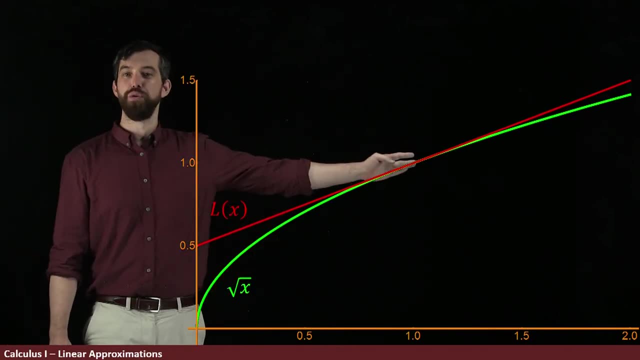 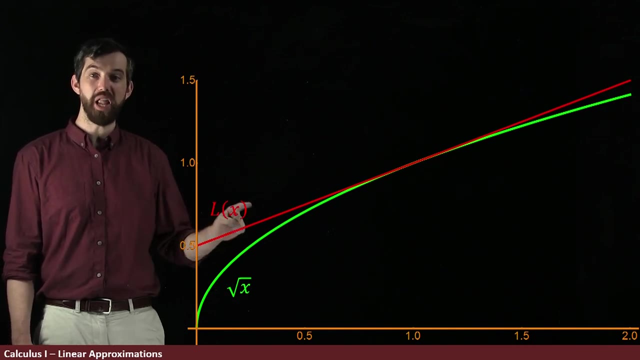 It's a really, really good approximation, at least in the case of this function sine of x. Let's do one more example Here I have the function square root of x And then I've taken the linear approximation. this tangent line stands for line here. 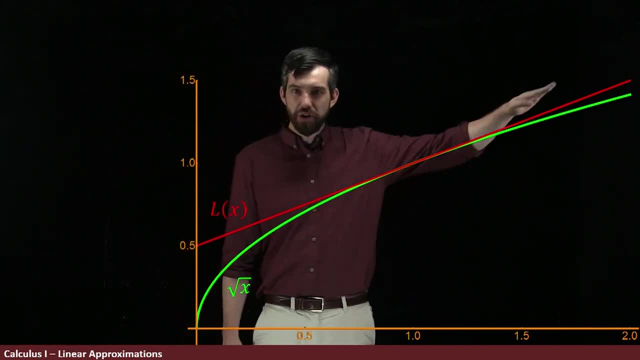 And I've done it at the value of x equal to 1.. So I've got this tangent line here And again it looks like a pretty good approximation at the value of 1.. And we could zoom in, And again it looks like a pretty good approximation at the value of 1.. 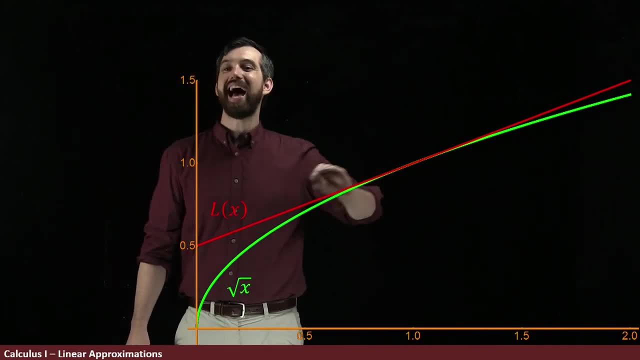 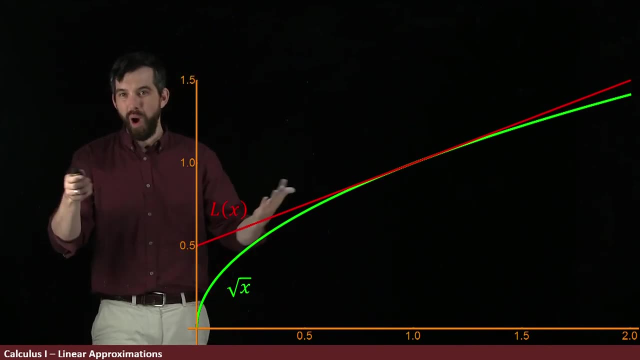 We could zoom in, zoom in, zoom in Until we had them basically exactly on top of each other. But sure, it looks like a good approximation. Now, the reason why I chose 1 is I know what the square root of 1 is. 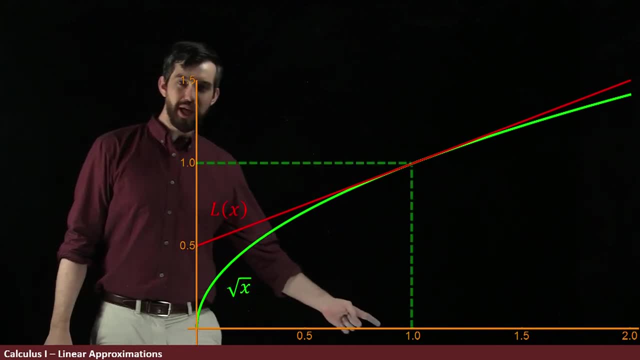 the square root of 1 is just 1.. I can do that pretty easily And indeed we could plug in the 1 here and we could get out the value of 1.. But you know what? I don't know how to do with my head. 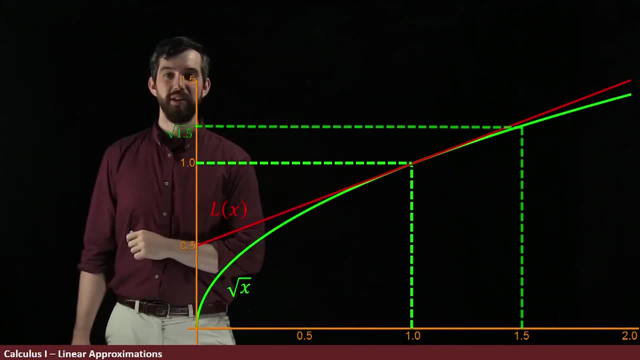 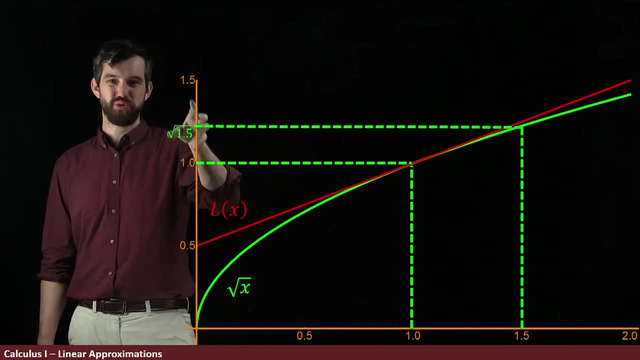 The square root of not 1, but 1.5.. I know it's 1.5 is my input. it comes over to here. There's some value- 1.5,. I could probably guess that it's in this region, but I don't know exactly what it is. 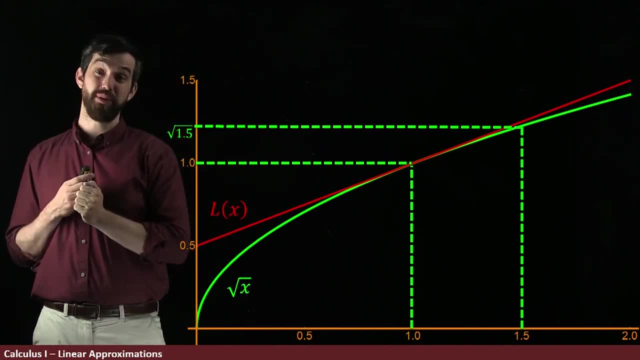 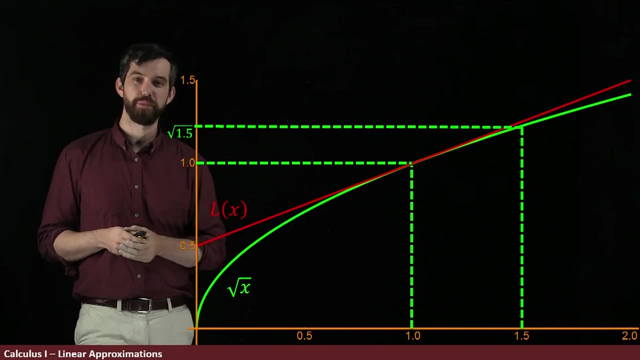 I don't know what this number is. Maybe it's got an infinite decimal expansion. So how should we compute this? How does the computer even compute the square root of 1.5?? One thing that I could do as an approximation is if I look at this tangent line and remember this tangent line was a tangent. 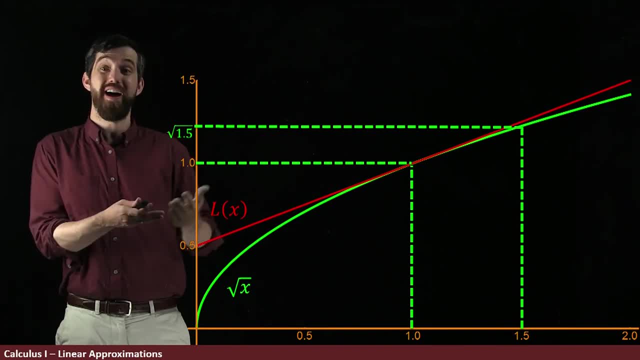 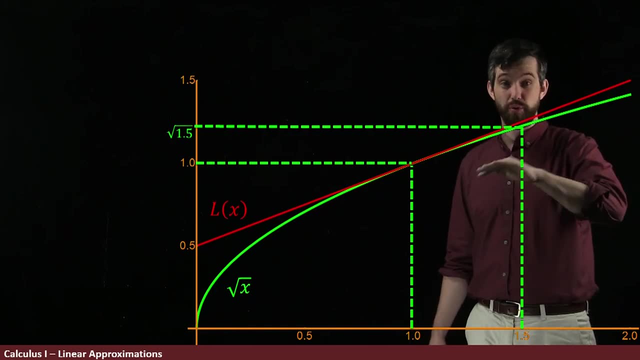 line at 1.. It's not the tangent line at 1.5.. 1.5 is a little ways away. So if I go over to 1.5, you can see that there's the green that's my square root of x, and that there's the red. 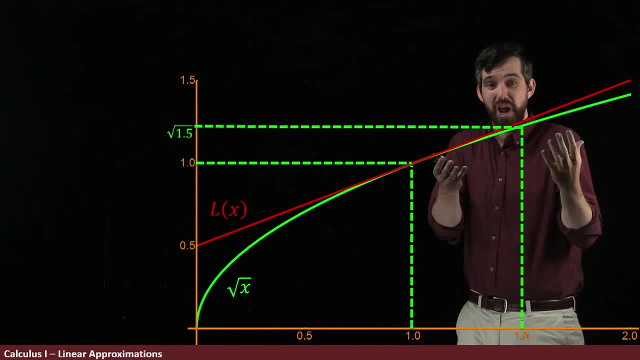 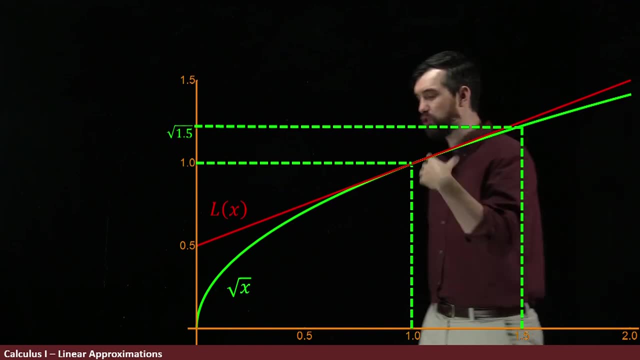 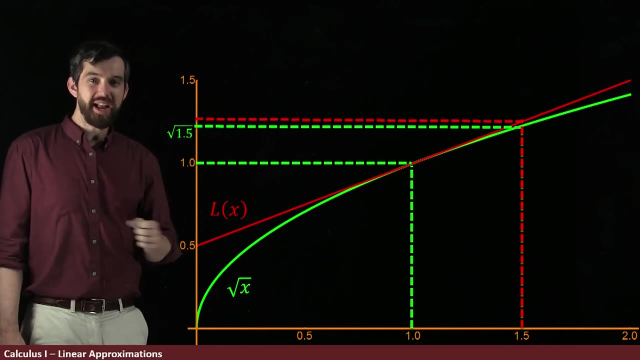 that's my line and they're pretty close but they're not exactly the same. but it's a good approximation, right, The height here on my tangent line of 1.5 and the square root of 1.5, they're pretty close So I could do an investigation of that. I could ask at 1.5,. 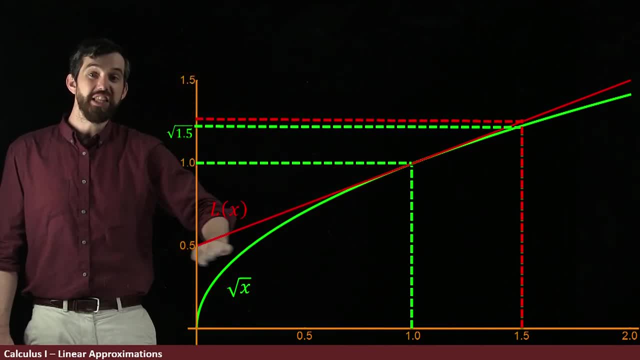 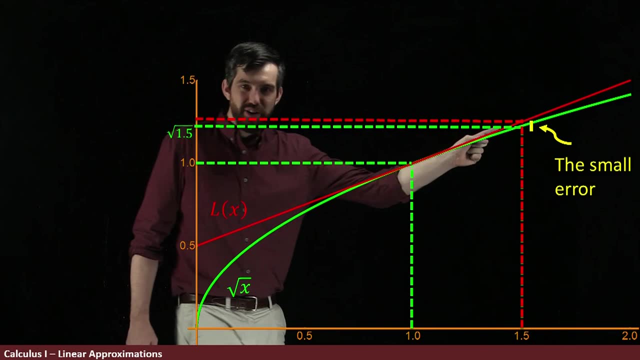 what is not square root of x, but this line, this tangent line. I could ask what is l of 1.5?? And yeah, they're a little different, but the error here, the difference, this little extra height, here it's really small. So our heuristic is this: 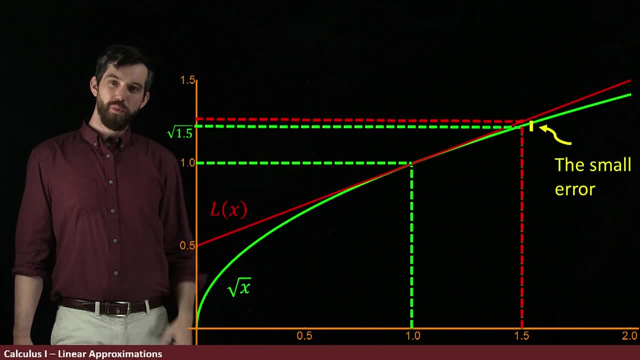 When I'm trying to estimate something like the square root of 1.5,, what I'm going to do is I'm going to compute the tangent line not at 1.5, but at a number I can actually compute, I know. 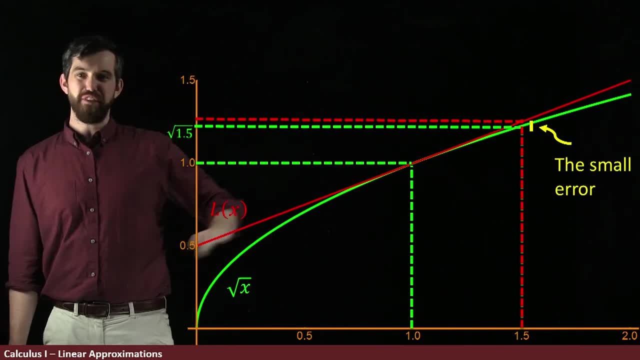 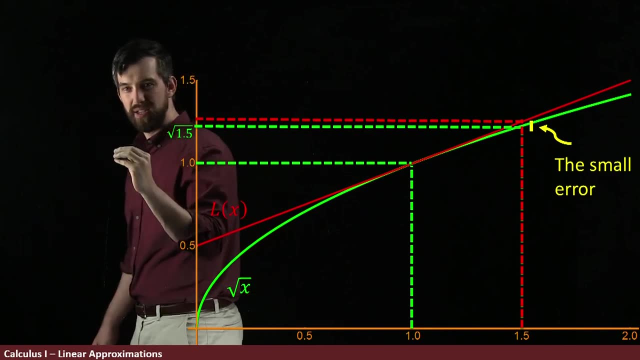 how to do the square root of 1.. And then I'm going to try to figure out what that tangent line is. I'm going to go along the line over to the 1.5, and that value is not going to be exact, but it's going to be pretty good. 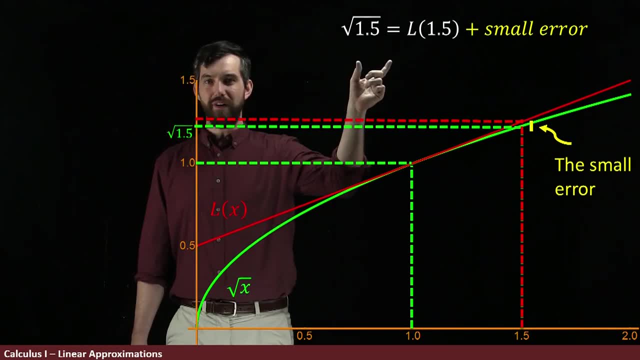 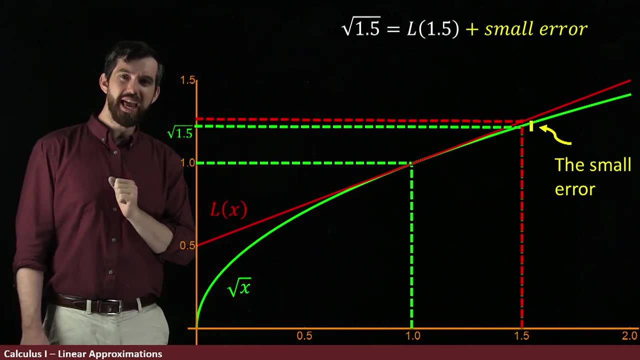 Another way to think about this is to say that the square root of 1.5 is whatever the line is at 1.5, whatever my tangent line is at 1.5, plus this small little error, In this case, where the tangent line is above the square root of x. the small error is a small. 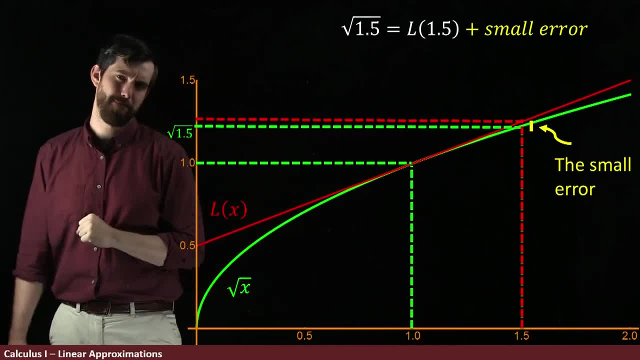 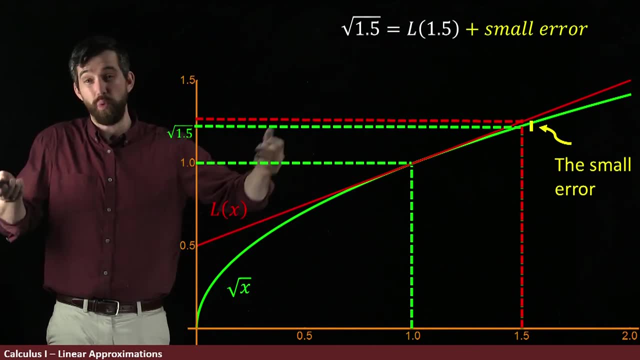 negative number. So the green is a little bit less than the red. And another way I can say it is if my error truly is small and I haven't justified outside of this graphical picture why it's a small. but if it truly is small, then I'd be able to say that the square root of 1.5 is approximately. 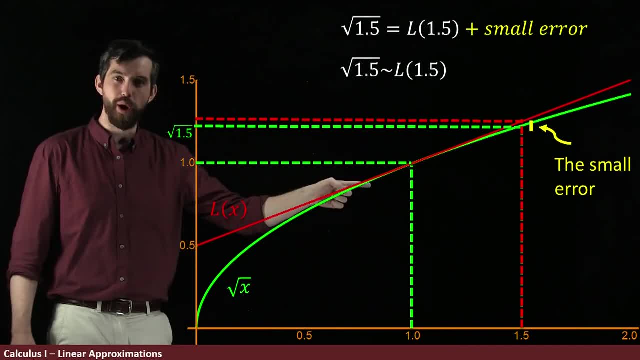 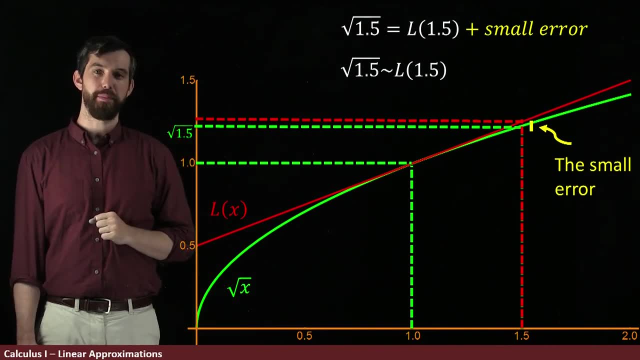 the same thing as the tangent line computed at the point 1, but evaluated over here at 1.5.. So let's try to figure out what is this tangent line. So that's our goal: The square root of 1.5. 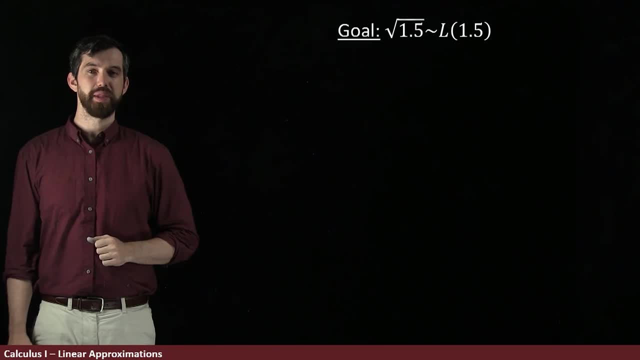 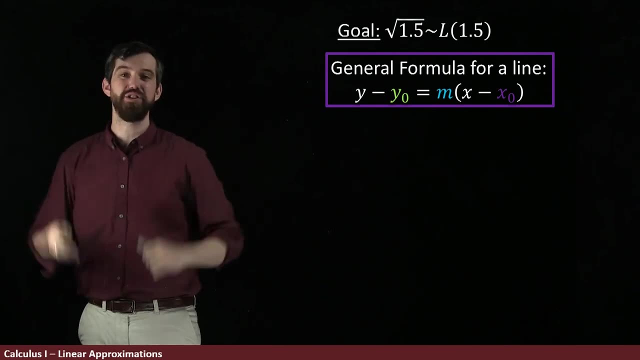 is the tangent line at 1, but evaluated at 1.5.. And I'm going to remind you first the general formula for a line. So any line at all, tangent line, secant line, any line, you just have to. 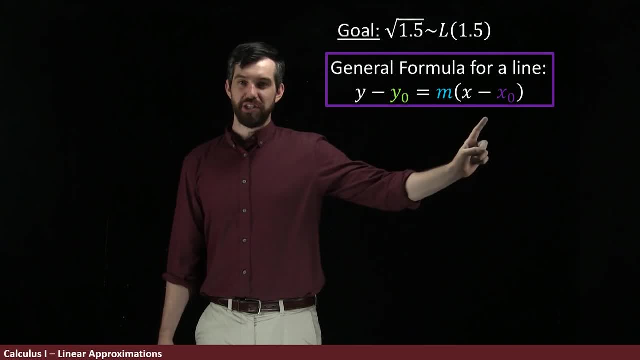 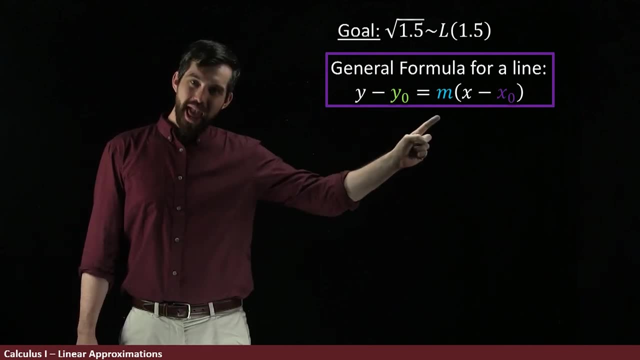 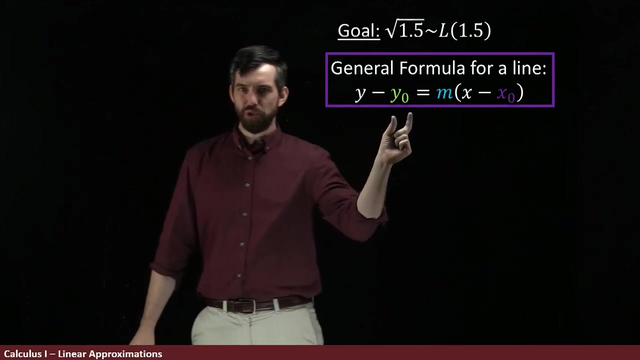 choose is going to have your y and your x as your variables. your y naught and your x naught as two starting points, and then your m here is as the slope. This is so-called the point-slope formula for a line. Sometimes people take this y naught and the m times x naught and they put it all: 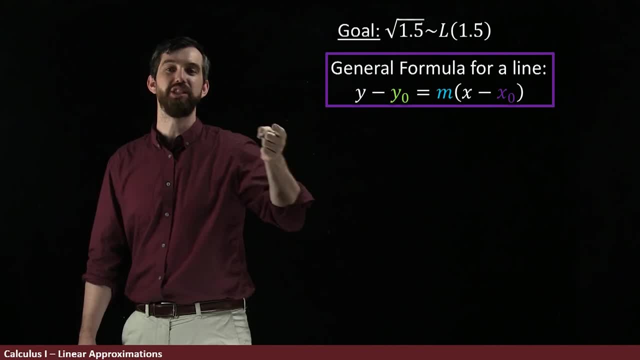 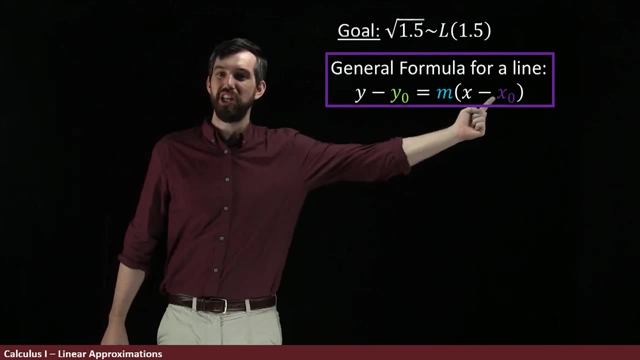 over to the right and then it's: y equals mx plus b, where b is the y-intercept. You can do that form and that's the slope-y-intercept form. but I generally prefer the slope-point form because I usually know two points: an x naught and a y naught. So let's try to do this for our 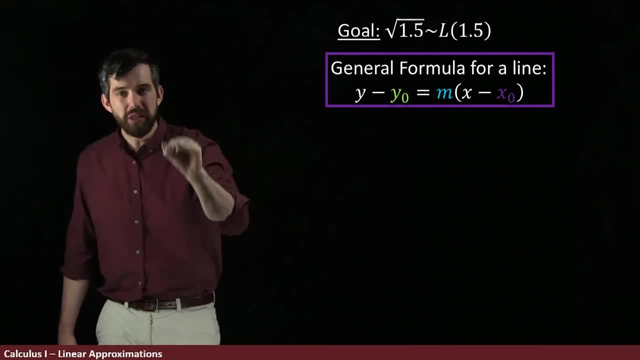 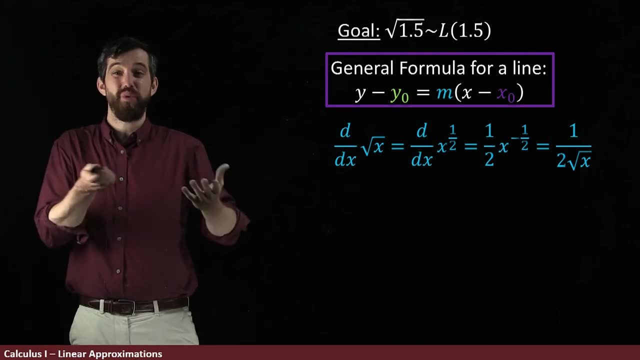 scenario. We want to figure out the m. The m is the slope and the slope is given by the derivative. So that's what I need to do: Derivative of square root of x. Easy enough. The only sort of weird trickery is to note that square root of x is really x to the power of 1.5.. I like it better. 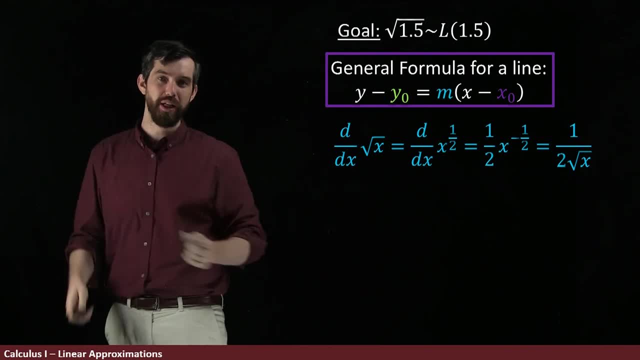 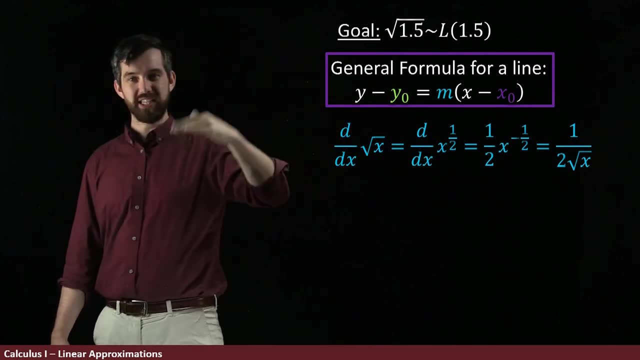 in the form x to the 1.5, because then I can apply the power rule x to the 1.5, I apply the power rule x to the 1.5. minus 1 is x to the minus 1.5.. That's why I have x to the minus 1.5.. And x to the. 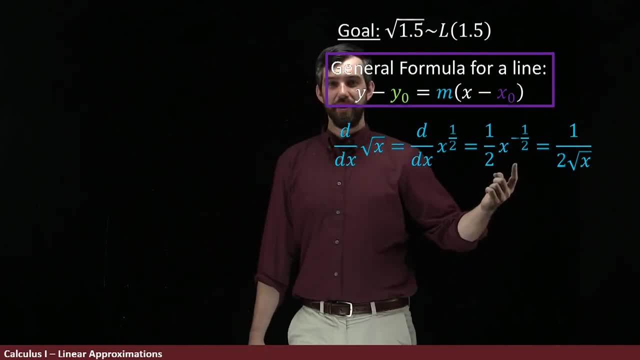 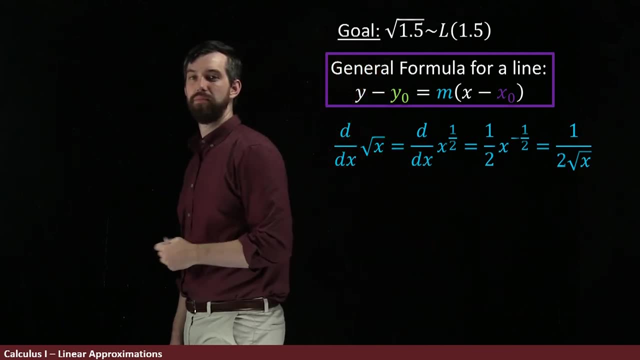 minus 1.5,. you don't have to do this, but it's nice to rewrite it. The minus sign means it's x to the half, but on the bottom, And x to the half is square root. So 1 over 2 square root of x. So 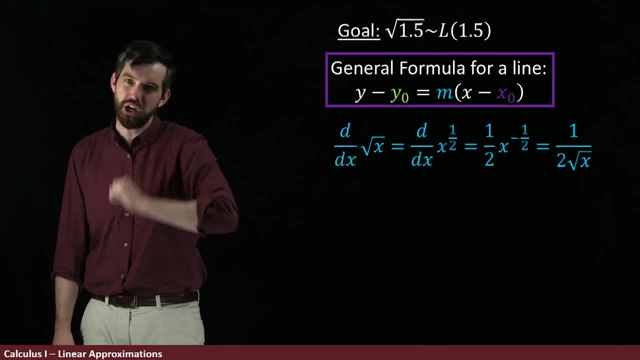 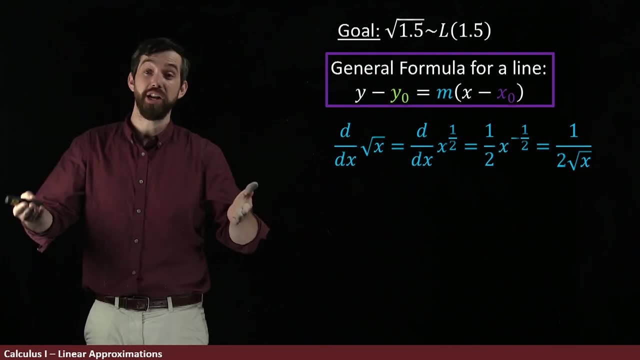 there you go. We've got what our slope is for all values of x And, in particular, what we're interested in is the point x equal to 1.. x equal to 1 means square root of x. The y naught here is: 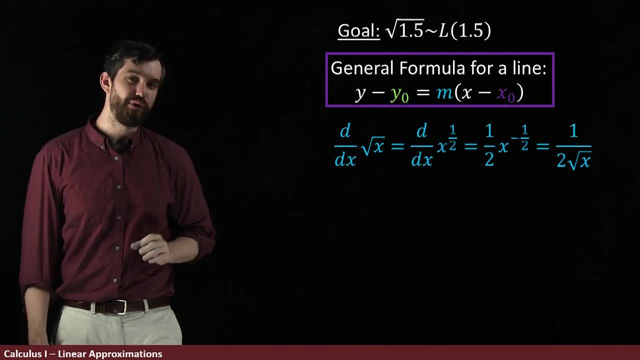 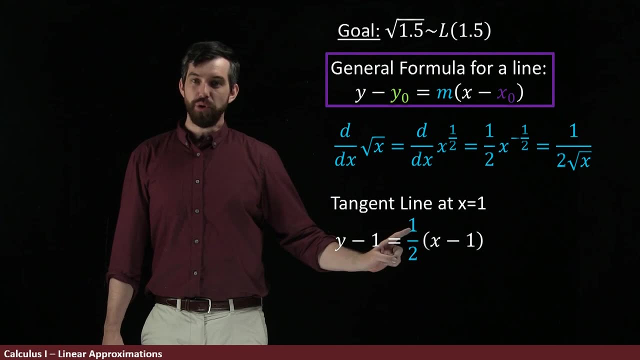 1.5.. And therefore, taking all of this into my general formula for a line, what I get is going to be: y minus 1, that's the square root of 1, is equal to 1.5.. That's the slope here of value. 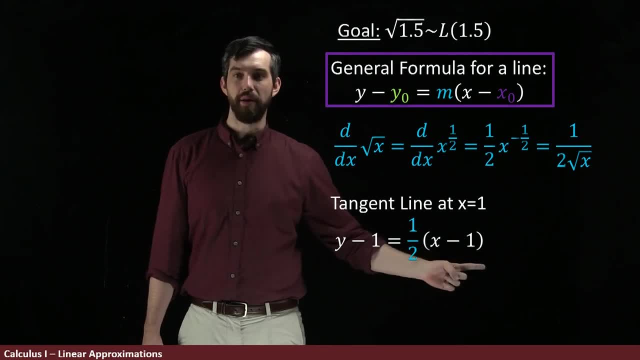 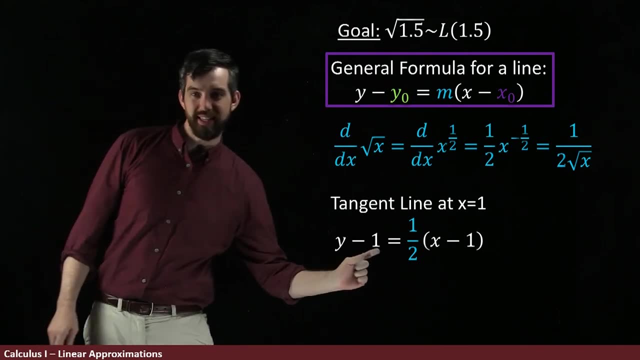 at x equal to 1.. x minus well, x naught is just equal to 1.. And so this is going to be my tangent line, And then, if I actually want to write it as a line, y equals something. I'll take this minus. 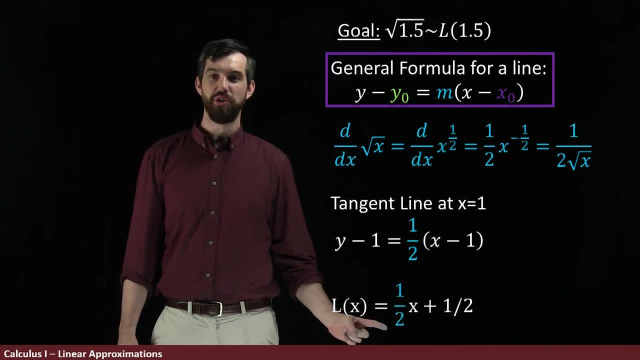 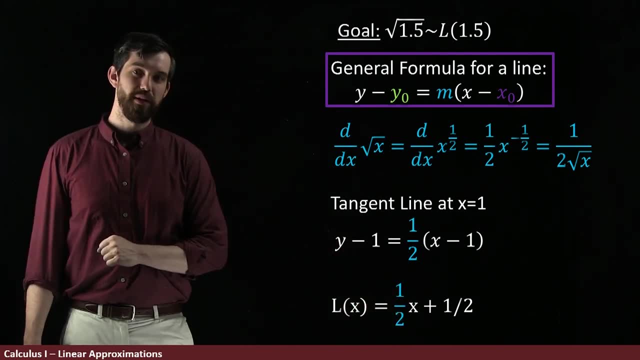 1. I'll move that over to the other side And what I get is: Lx is equal to the mx plus b4.. The slope intercept form: 1: half x plus a half. This, by the way, when I was doing my graphing. 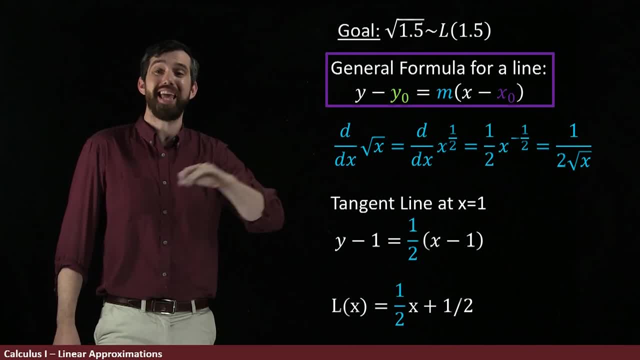 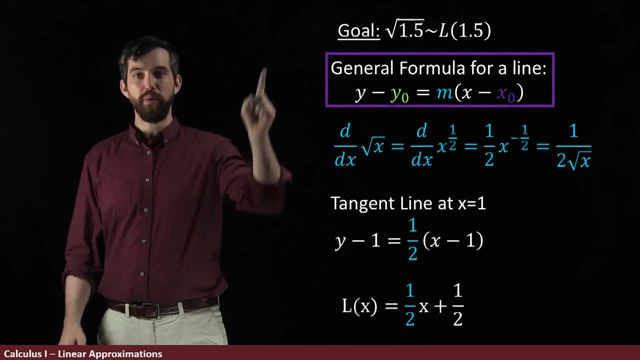 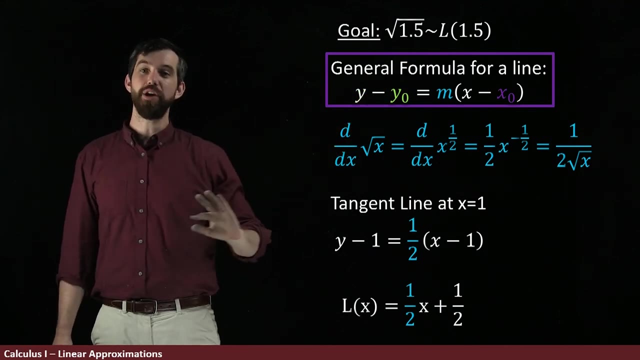 beforehand. I figured out this particular equation first, And that's how I was able to draw the tangent line going on top of the square root of x. Now we've got L of x for all values of x. But remember what our goal is. Our goal was: the square root of 1.5 is about L at 1.5.. So let's get rid of. 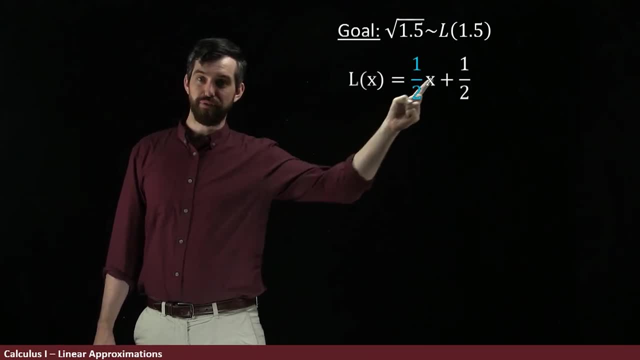 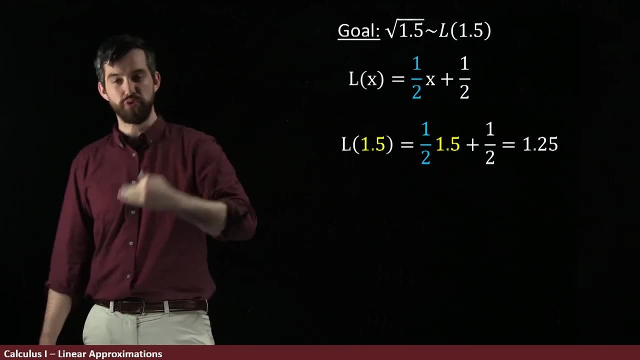 our calculations. I've got this L of x And what I want to do is figure out L of 1.5. And I want to plug in 1.5.. So this is going to be: 3 halves divided by 2 is 3 quarters: 3 quarters and a half. 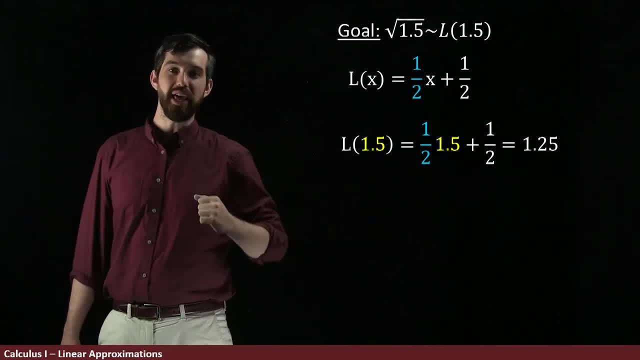 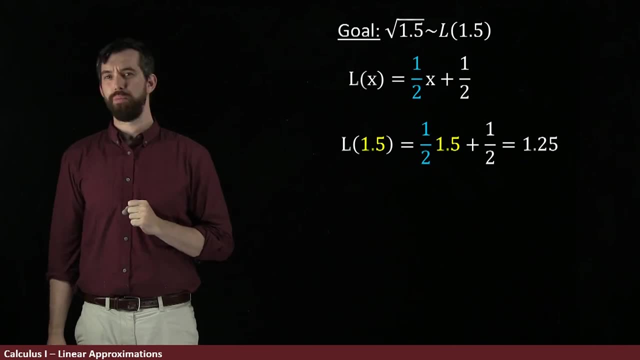 is 1.25.. So that's my claim. My claim is that square root of 1.5 is about- not exactly, but about- 1.25.. Now I'm going to actually go on the calculator here and spit out exactly what the 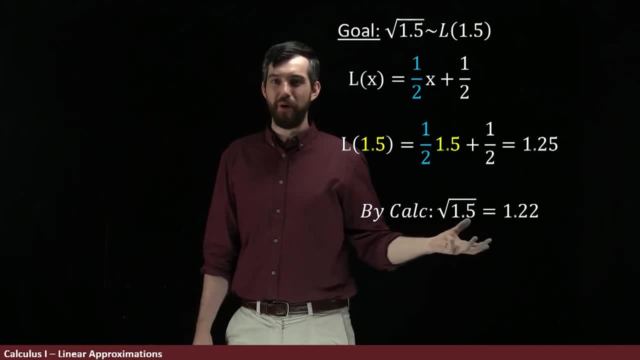 number is at least two decimal places. I could compute that the square root of 1.5, according to my calculator, is 1.22.. Not so bad, So I'm going to go on the calculator here and spit out exactly. 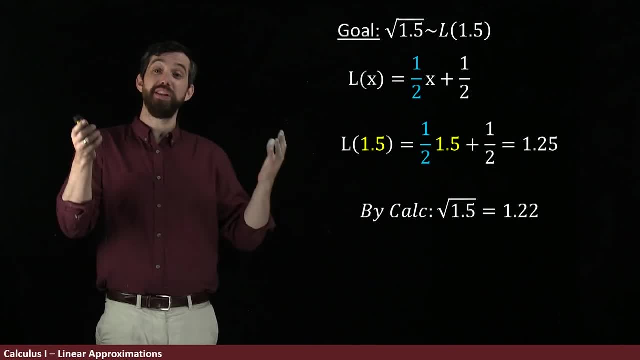 what the number is, at least two decimal places. So that's my claim. My claim is that square root of 1.5 is about, not exactly but bad. 1.25,, 1.22, they're close, They're only a little bit away. Indeed, if I go back to my original, I have the: 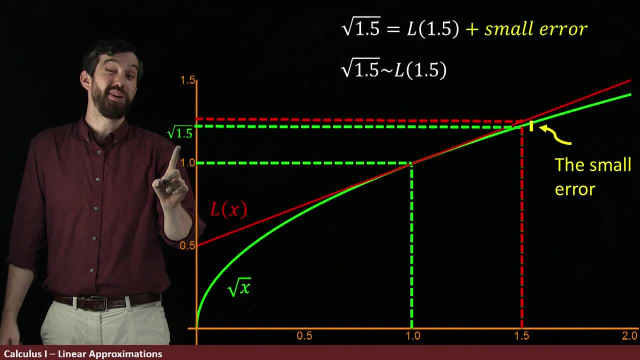 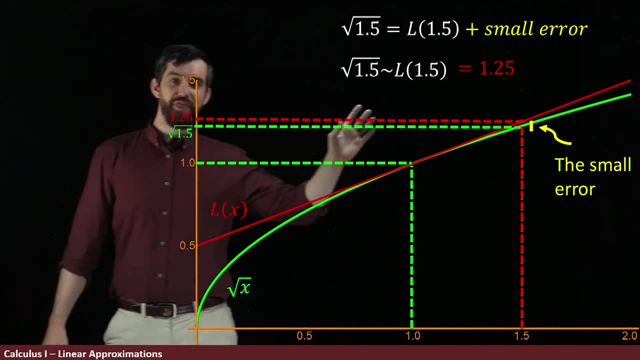 square root of 1.5.. That was the green here, which the calculator tells me is 1.22.. But by our approximation what we can see is that 1.25, that is what my tangent line at the value of 1.5 is. 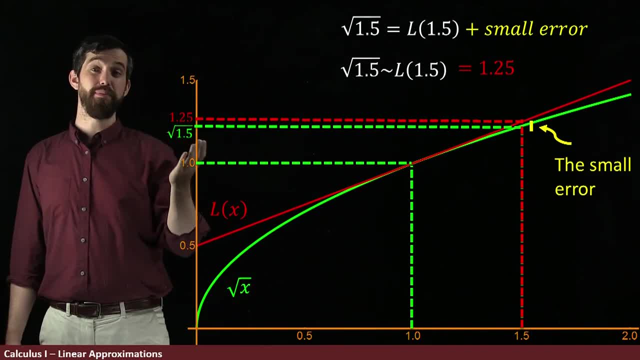 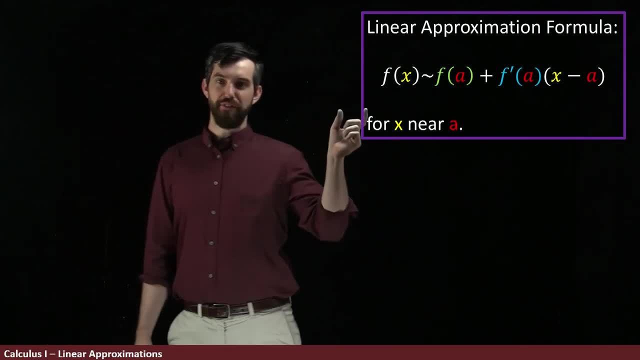 going to be. It's 1.25, and it's a pretty close number, Not so bad. So, in summary, I'm going to go ahead and write this down. So, in summary, the grand linear approximation formula is that, if I'm